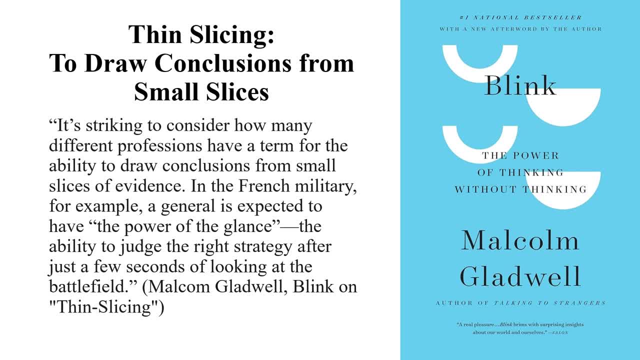 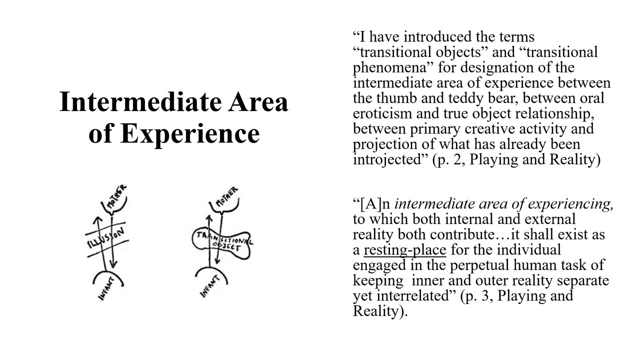 In the French military, for example, a general is expected to have the power of the glance, the ability to judge the right strategy after just a few seconds of looking at the battlefield. We move now to Winnicott, who draws our attention to the intermediate area of experience. 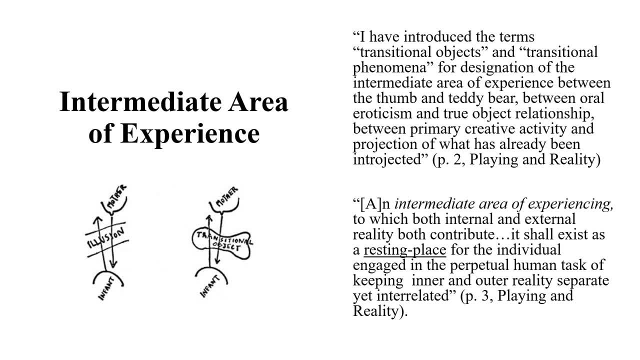 between the subjective and the objective, And I quote from Playing in Reality. I have introduced the terms transitional objects and transitional phenomena for designation of the intermediate area of experience between them, the thumb and the teddy bear, between oral eroticism and true object relationship. 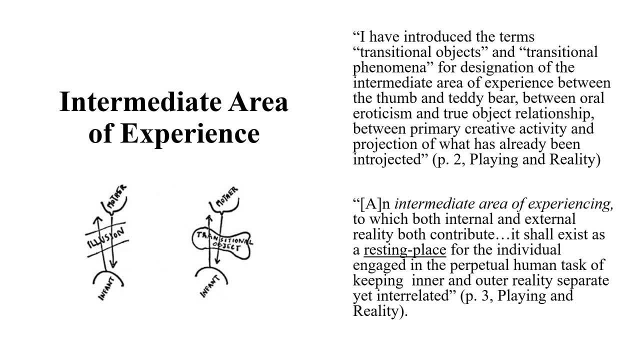 between primary creative activity and projection of what has already been interjected, And I continue- an intermediate area of experiencing to which both internal and external reality both contribute- It's interesting- shall exist as a resting place for the individual engaged in the perpetual human task of keeping. 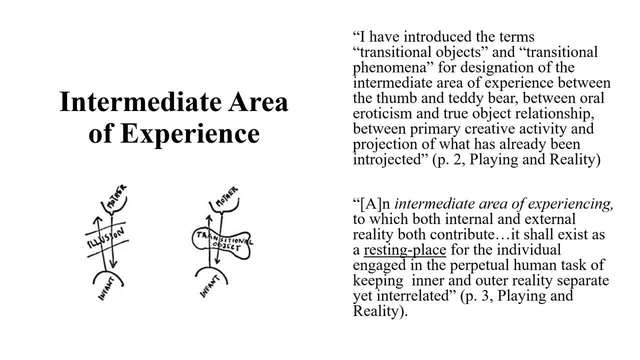 inner and outer reality, separate yet interrelated. So we have a mother and an infant and we have this association with this blankie engaging with the mother. The baby associates over time this object with the mother and when they're left away from the mother, they can hold the blankie or teddy bear. 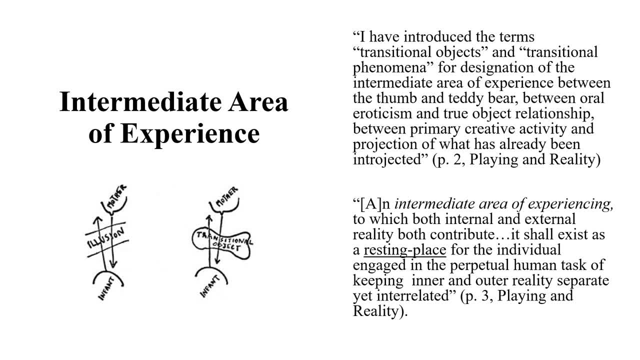 Welcome This objective piece of textile and regulate their experience by thinking of the mother, the symbol of the mother, while holding the teddy bear. It's both a textile and my teddy, my blankie, what Winnicott refers to right as the first possession. 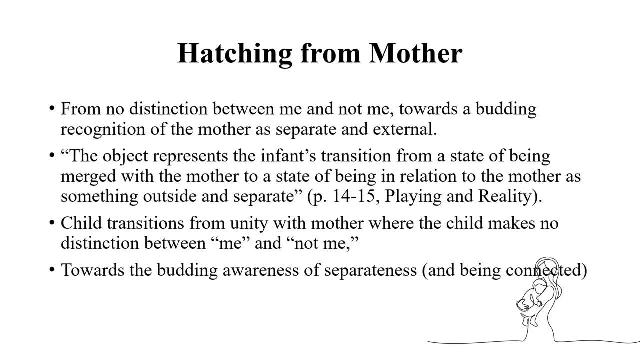 Hatching from the mother, from no distinction between me and not me, towards a budding recognition of the mother as separate and external. the object represents the infant's transition from a state of being merged with the mother to a state of being in relation to the mother as something outside and separate. 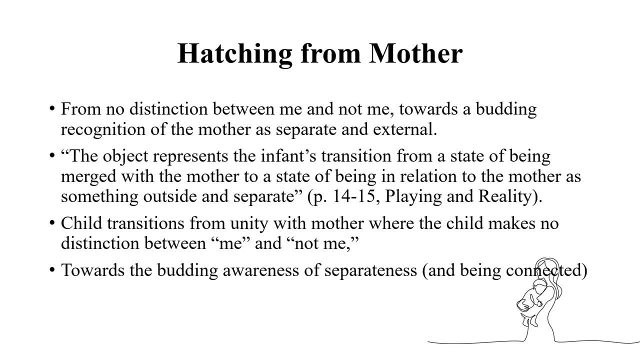 The child transitions from unity with mother, where the child makes no distinction right between me and not me- Oneness, and then a hatching towards the budding awareness of separateness and then with that, as being connected in a new way: The infant and the mother, and the mother is represented symbolically in the absence of her presence. 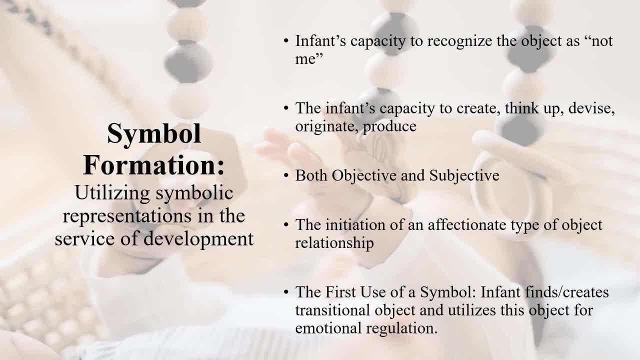 So we have this profound process in the first year of life where the child is able to use the infant, right in the first year, a symbol in the service of development, okay, The infant's capacity to recognize the object as- not me, as- separate, and they could throw it up in the air and push it up against the wall, stomp on it. 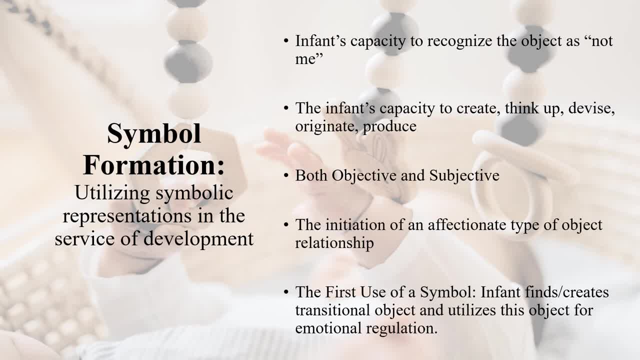 With their feet. it's something they can engage as a living aspect, and with it comes the infant's capacity to create, think up, devise, originate, produce and, once again, right, it's both just a piece of woven textile and it's my blankie. the subjective aspect, the creative aspect. 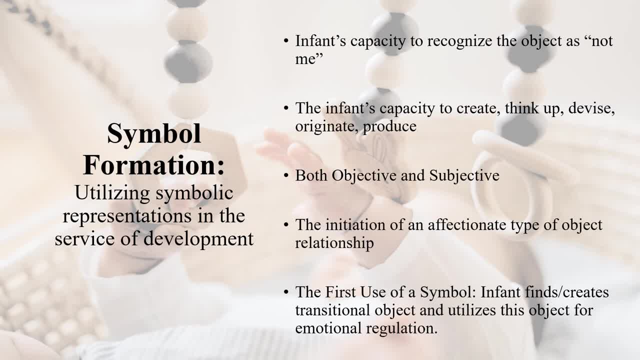 The initiation of an affectionate type of object relationship and, as we've reported, right this first use of a symbol, the infant finds creates this transitional object and utilizes this object right to transition from a state of tension, of disappointment, of being unsettled, undisregulated and holding the blanket. 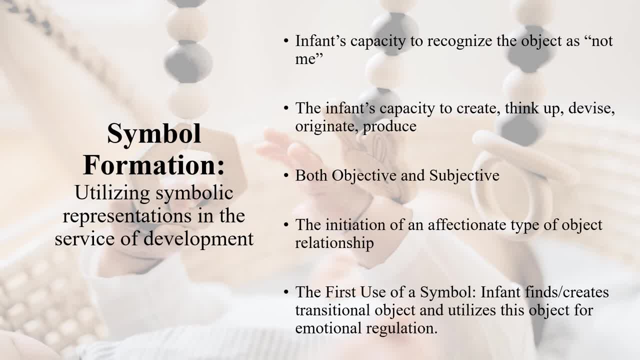 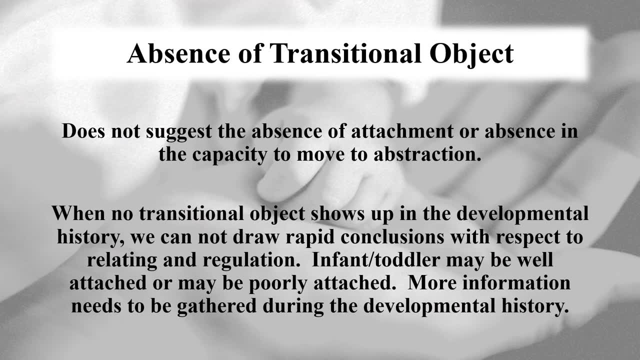 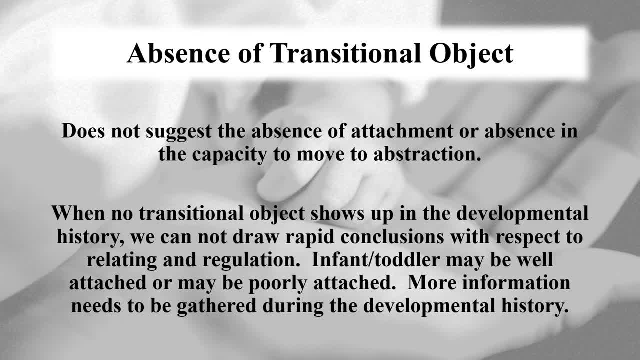 Or absence in the capacity to move to abstraction. Okay, when no transitional object shows up in the developmental history, We cannot draw rapid conclusions with respect to relating and regulation. The infant-toddler may be well-attached or may be poorly attached. 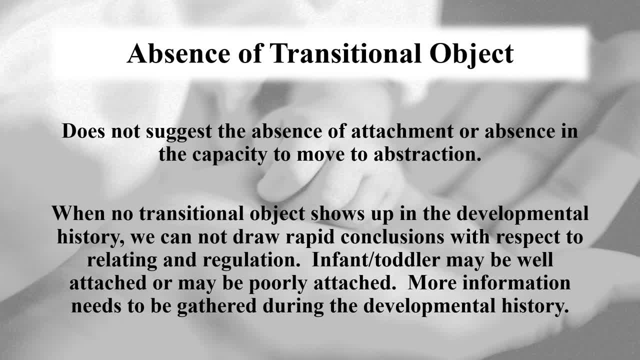 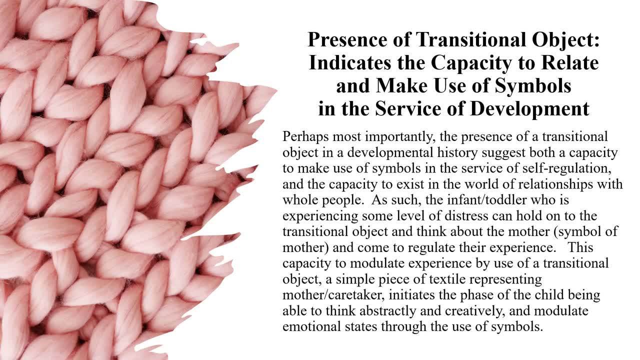 More information needs to be gathered during the developmental history, But what we can see is when we have the presence of a transitional object, essentially a creative way for the infant to solve the problem of being moved away from the mother at night and have to sleep through the night in a separate room in a crib by themselves. 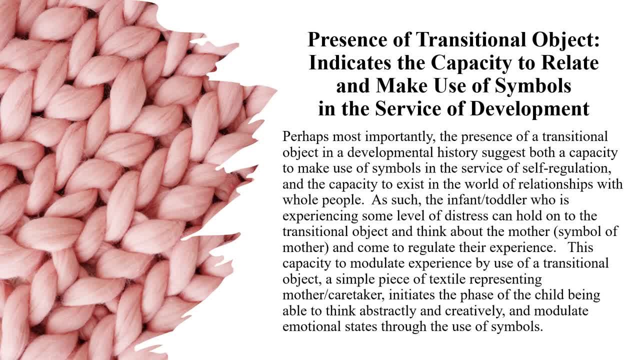 This is their solution to that problem. So the presence of transitional object. it indicates the capacity to relate and make use of symbols in the service of development. Perhaps most importantly, the presence of a transitional object in a developmental history suggests both a capacity to make use of symbols. 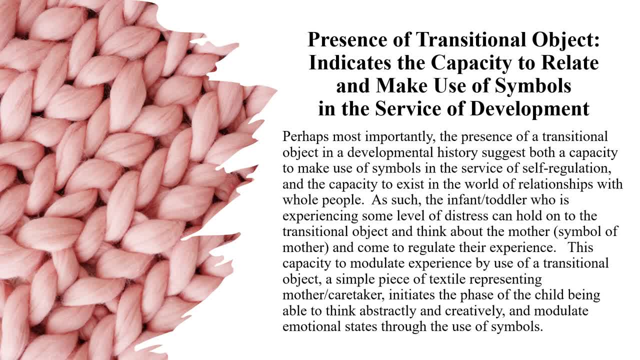 in the service of self-regulation and the capacity to exist in the world of relationships with whole people. As such, the infant-toddler who is experiencing some level of distress can hold on to the transitional object And think about the mother, the symbol of the mother. 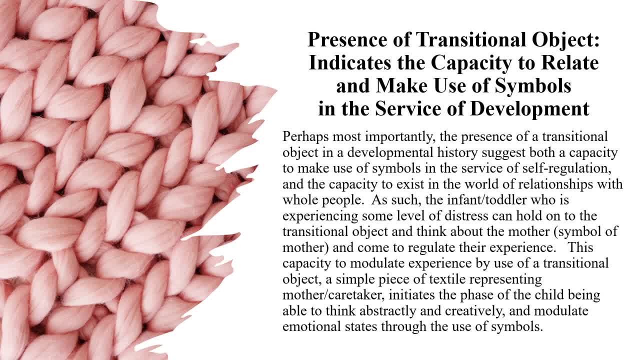 and come to regulate their experience. This capacity to modulate experience by use of a transitional object, a simple piece of textile representing mother caretaker, initiates the phase of the child being able to think abstractly and creatively and modulate emotional states through the use of symbols.